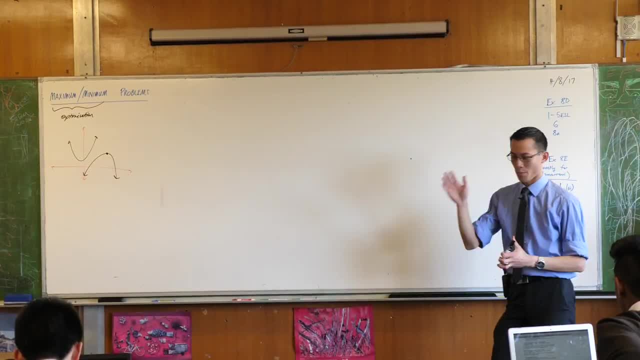 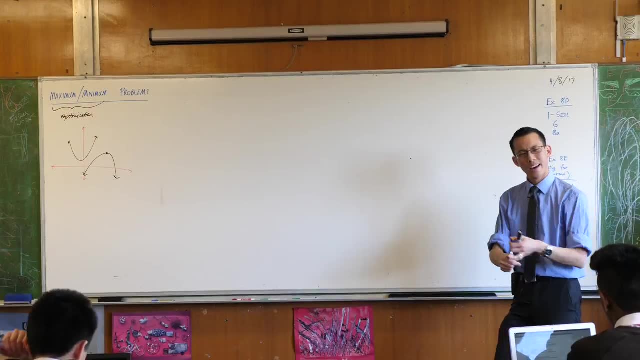 that would be equally easy to find. All I need to do is find out where that middle spot is, and off I go. There's the value that will give me the minimum, And there's the actual minimum itself. Okay, Now, when we're solving quadratic equations, there are three techniques that we use. 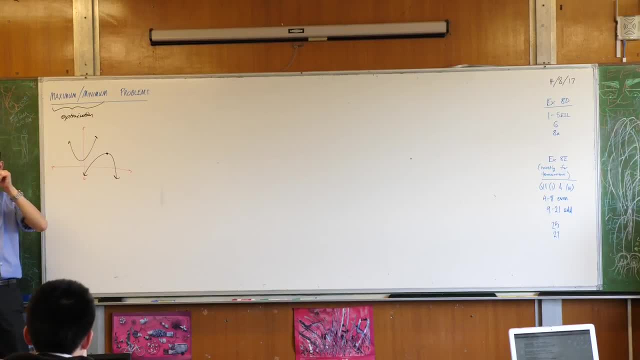 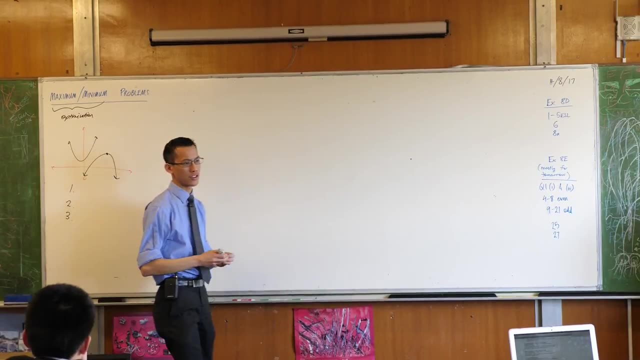 or three techniques that you can use which are exactly alike to this max-min problem, Right? So the three techniques are suggestions. If you tried to solve a quadratic equation, what could you do? What's the simplest method you could use? You can factorize. 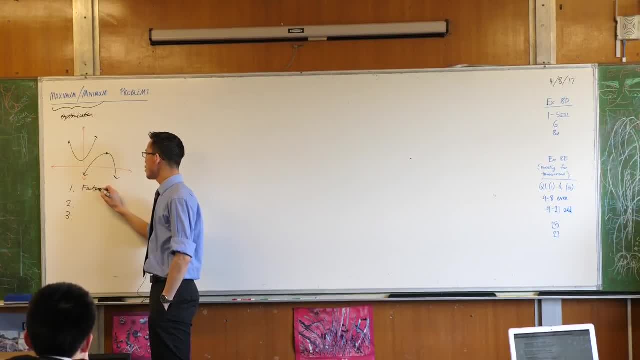 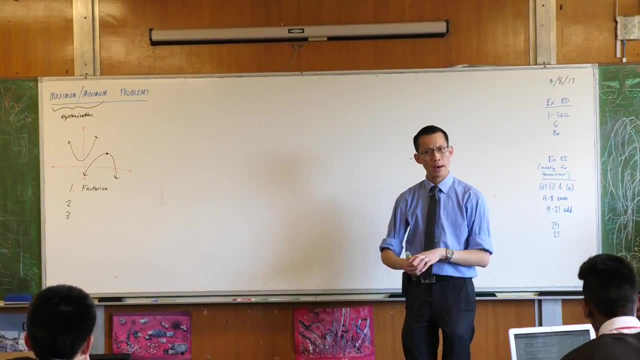 right. So when you factorize a quadratic equation then you say, oh, I've got two factors. make either of them zero and you solve the equation. But you wouldn't make them zero to find a maximum or a minimum. If you factorized, what would you do with? 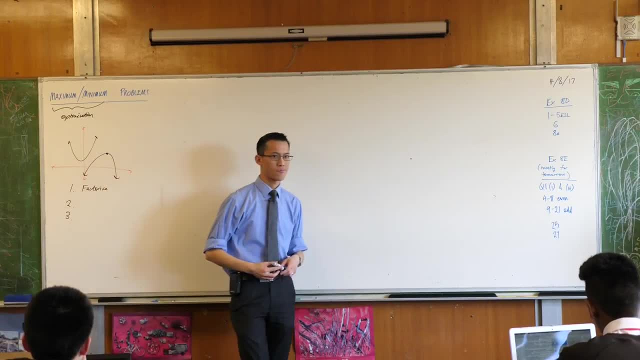 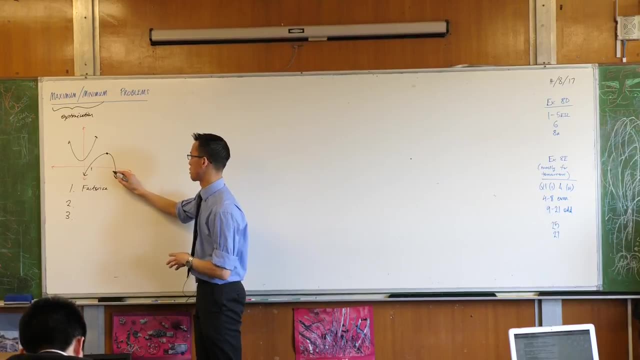 that information to get to a maximum or a minimum Like: suppose I factorize and I found that the factors are x minus one and x minus- what does that look like, I don't know? eight or something like that: X minus one, x minus eight. So then what do I do with that? 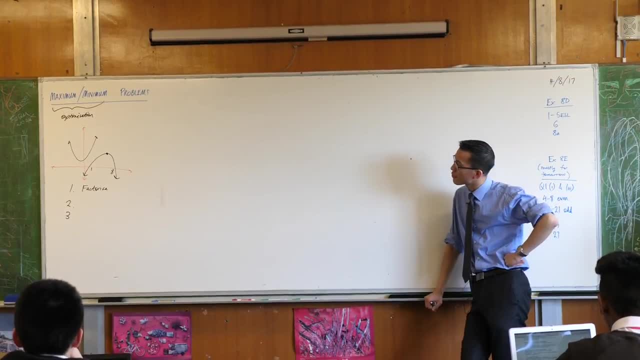 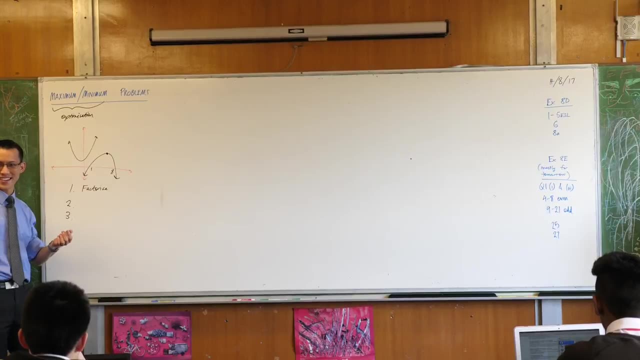 to find the maximum- Yeah, The second number minus the first number, and then divide it by two and go from the first number. Alright, I think that was a really accurate and complicated way to say: let's take the answer, Let's take the average right, Let's go halfway. Let's go halfway. Don't worry, it's my job. 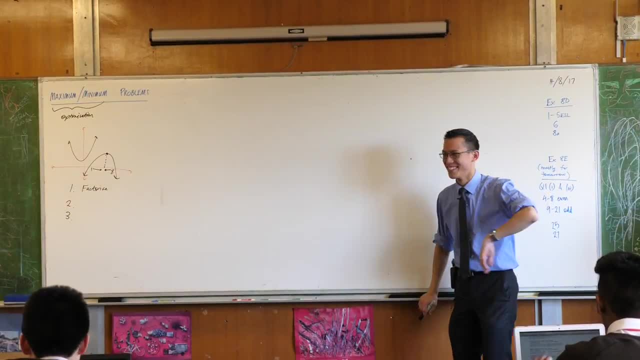 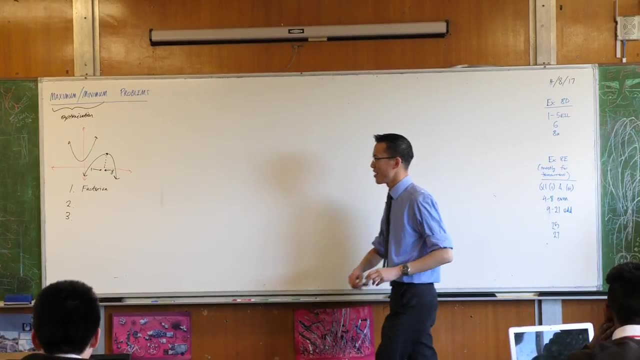 to do this, so you get a pass. okay. We could say: don't quit your day job, but you don't have one, so it's okay. What do we do? What do we do? We factorize and we use the factorization. 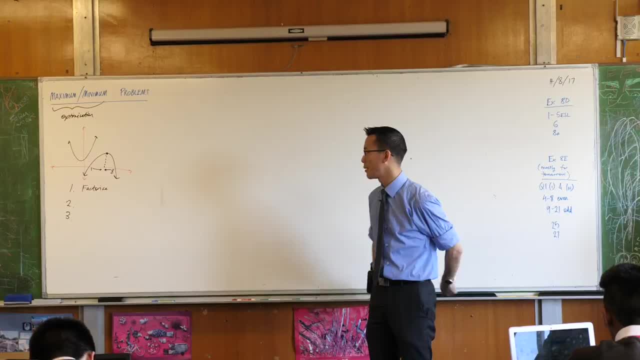 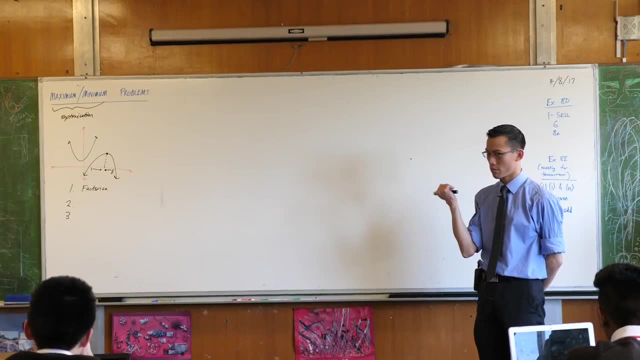 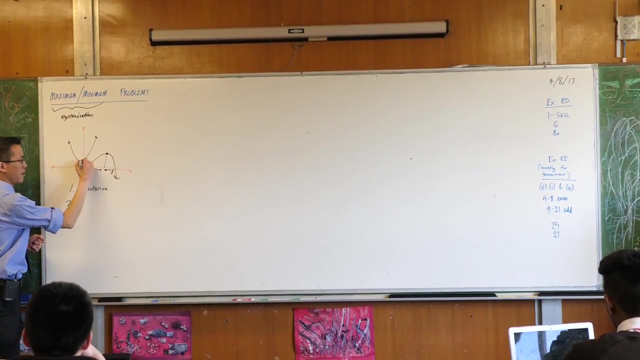 to say: well, the factorization gives me the roots. now I can go halfway. However, often you cannot factorize right For a variety of reasons. So what do we do in such cases? Quadratic formula: Okay, we can go to the quadratic formula. Now, if I want to find the middle, the vertex, 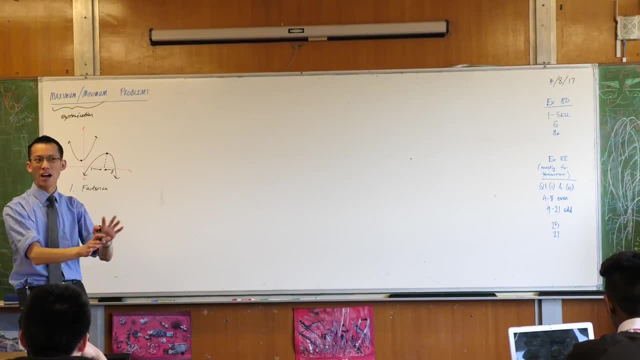 here the vertex. there I can go to the quadratic formula, but it's a bit unnecessary really, because there's something simpler that gets me straight to the thing I want. What is it, Rick? You had your head up. I don't know. 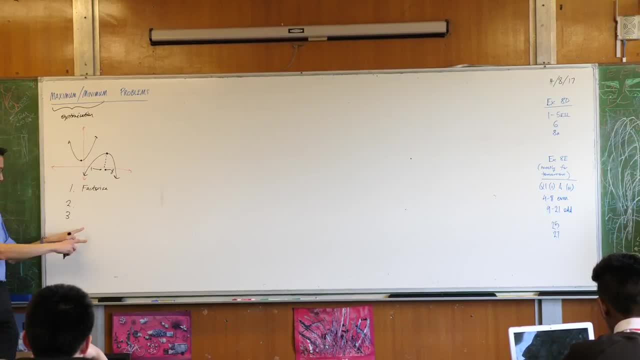 You were just stretching, Eric. We complete the square root. I will come to completing the square root. That'll be number three, because we haven't mentioned that yet. But to use the formula, I don't need to go like all the way through. 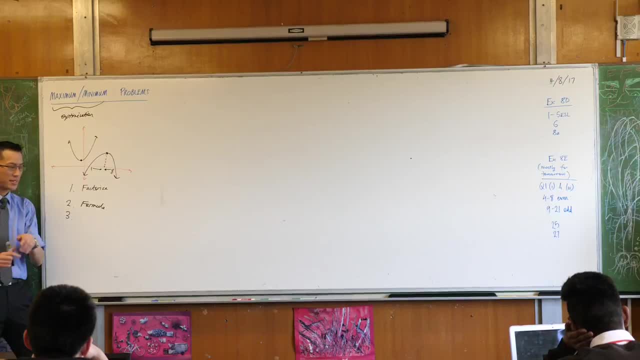 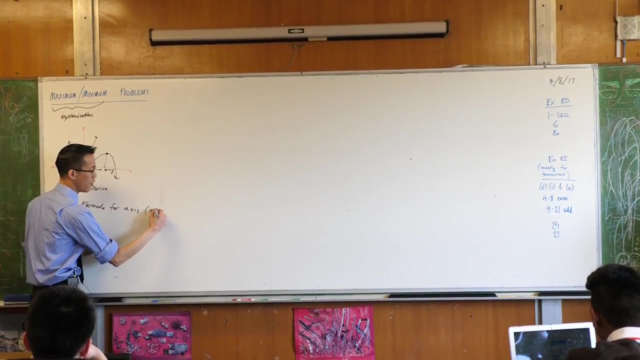 the whole square root of blah, blah, blah, blah, blah. yes, All I need is not the formula for the roots, I just want the formula for the axis, The axis of symmetry I can find as just the first part of the quadratic formula. See, there, it is right. The rest of the formula. 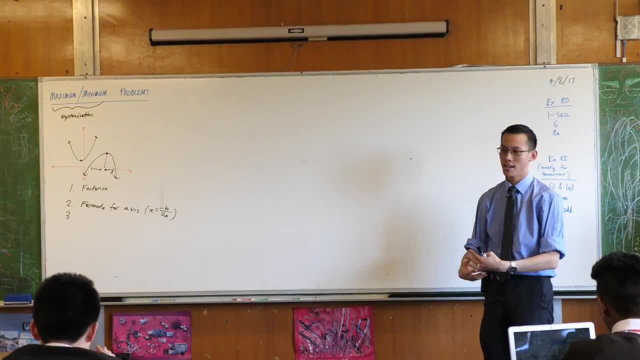 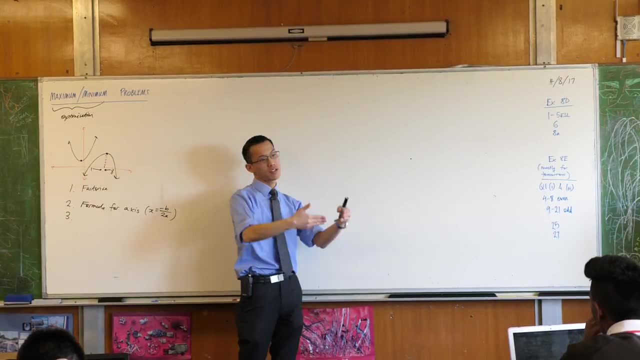 plus or minus the square root of b squared minus 4ac, all over 2a, is to give you the roots. But if what you really want is that guy, you don't need the roots. The roots are actually just a stepping stone to get to the vertex which gives you the real max or min. So we've 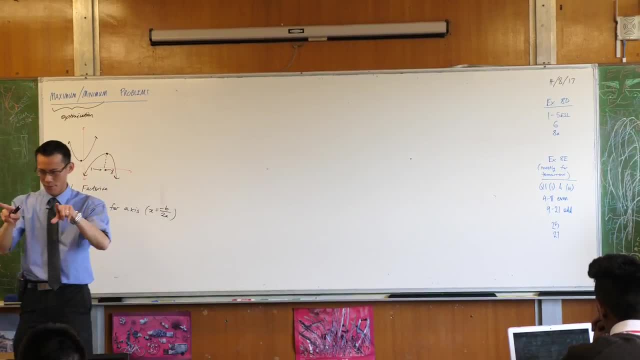 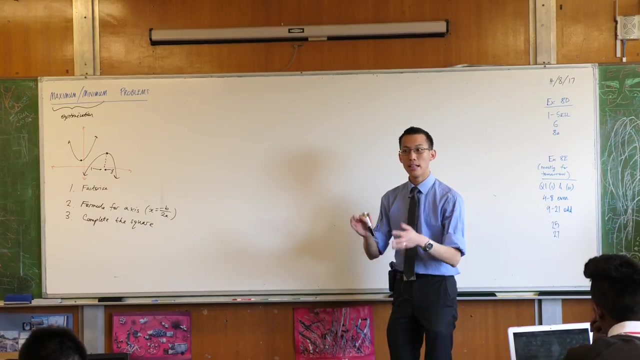 got factorization, we've got the formula, but for the axis, not for the roots. And lastly, as was suggested, we could complete the square. That's the other way that we can solve a quadratic equation. That's the mechanism for finding the max or the min. Let's have a look at some examples. 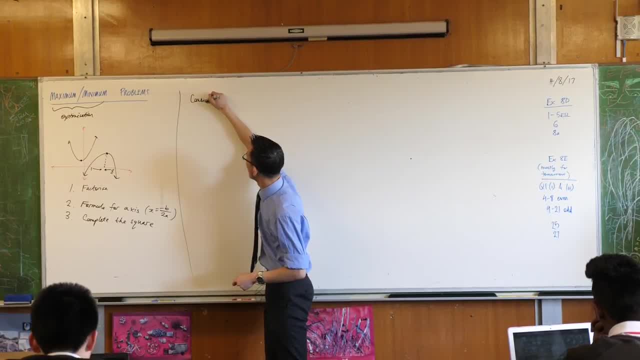 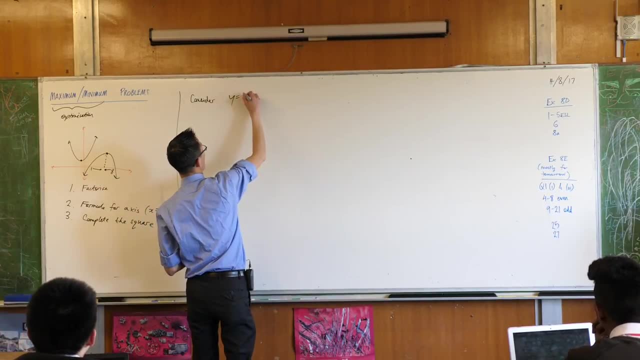 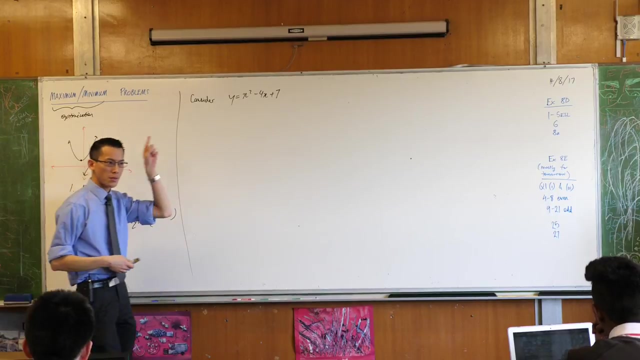 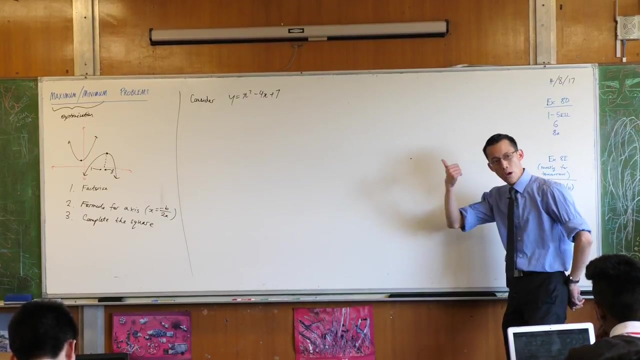 of each of these. okay, Consider, Okay, let me give you a function, Excuse me, Right? so when you have a look at this guy, we had a look at factorization before. You guys are super good at factorization, so I'm not going to labor the point. When you have a look at 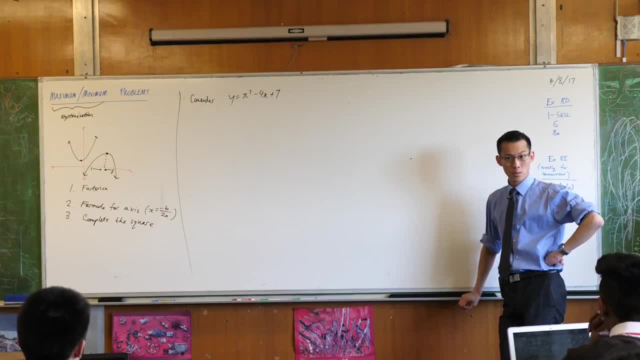 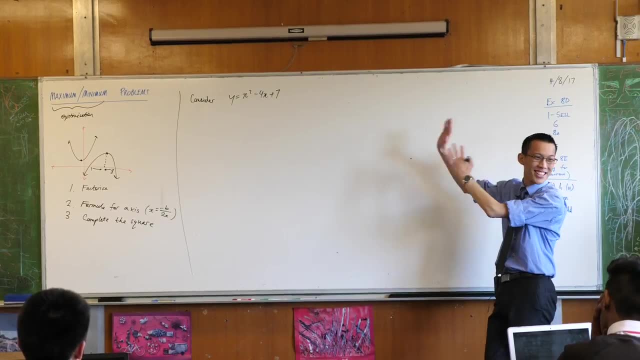 this. there's kind of a reason why I'm doing this. There's a reason why I'm doing this. There's a clue. by the way, that don't bother factorizing. Can anyone tell me what the clue is? It's the seven, right? What kind of a number is seven, Prime Jerks? Okay, so it doesn't. 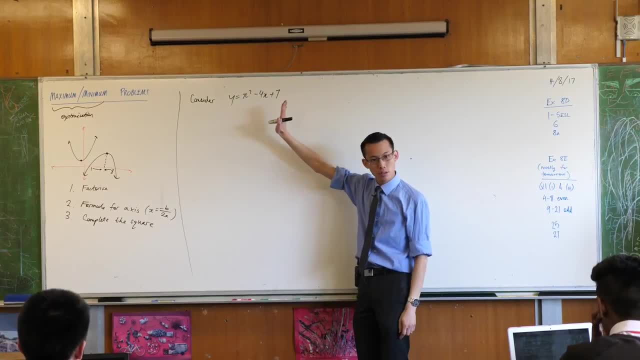 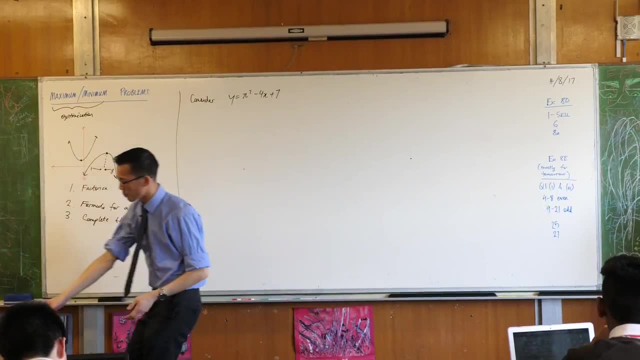 want to factor up into nice and neat pairs. So therefore, I'm not even going to bother. I'm going to choose one of these when I'm actually solving the problem Now, because I'm trying to illustrate this to you. let's just do both, okay. So method number two: 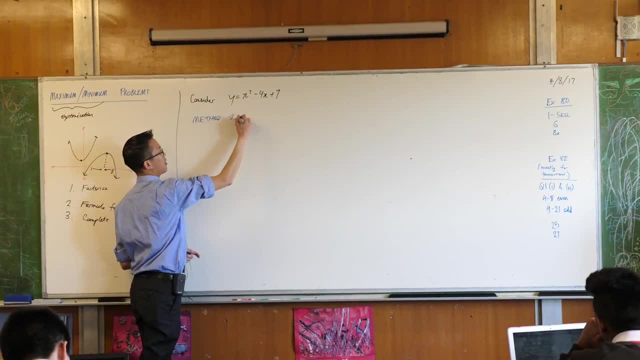 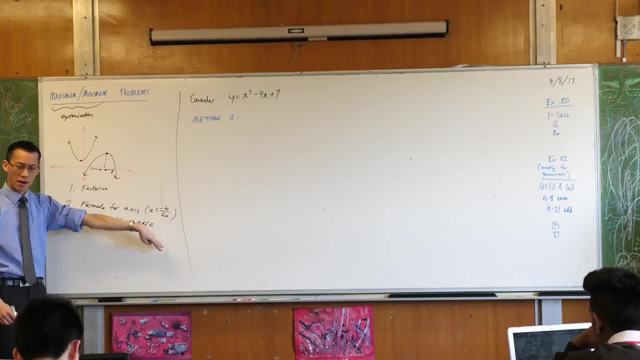 method two: let's go ahead and find the axis of symmetry. Okay, Now please don't just launch into this, because x is equal to a number, is? it could be anything. It could be a point on the curve, it could be an intercept, it could be who? 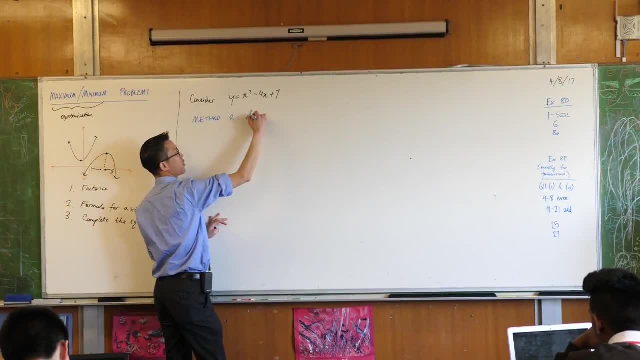 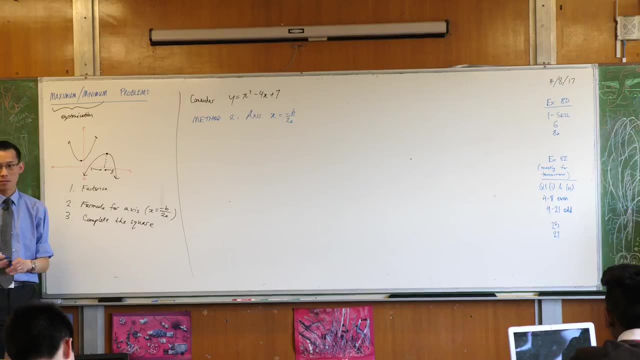 knows what it is. So when you're saying this, please tell me what you're actually calculating Like. so I'd be happy for you to skip the minus b on 2a and just go straight to the numbers once you feel confident to do that. but we're just starting off with this, so 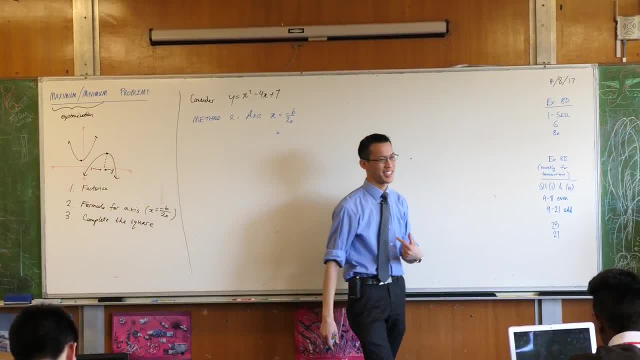 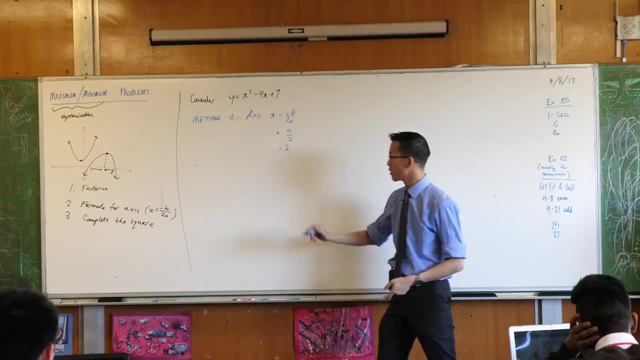 I'm going to write it down anyway. What is minus b on 2a? in this particular example, 4 over 2.. So I have an x value. Now, this is not, by the way, am I looking for a max. 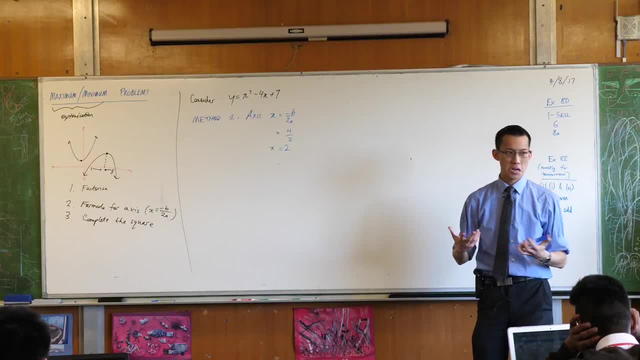 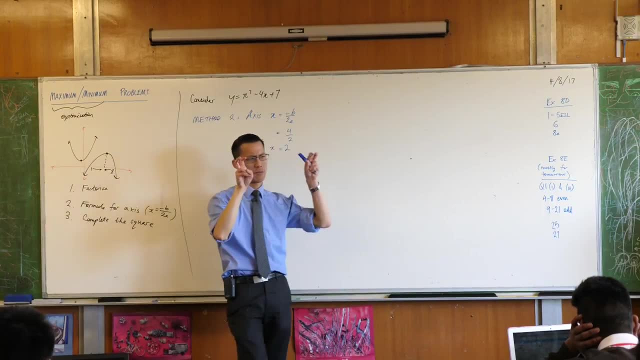 or a min. The only thing that makes sense for this question is a minimum, because it's going to be concave up, so the question of what's the maximum doesn't really have any meaning for this particular equation. So this tells me where I'm going to find the minimum. 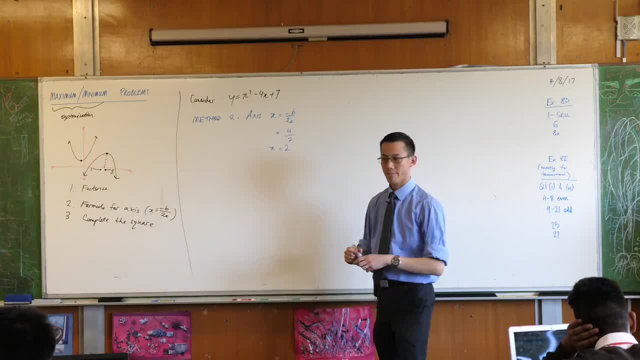 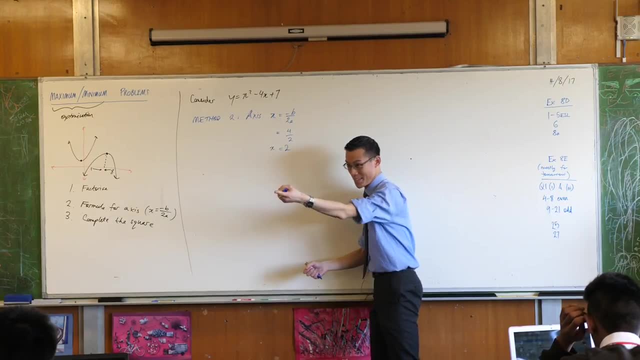 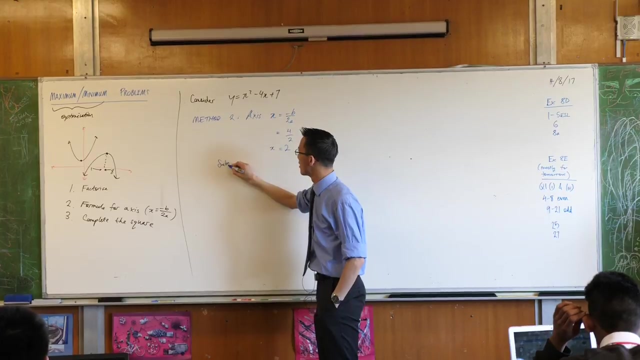 but it doesn't tell me what the minimum is. How do I do that? Find the y? I'm going to Table Whoa Again, a really complicated way to get the answer, but it might be simple just to substitute, right, I can take this, I can pop it into my original equation. We're just 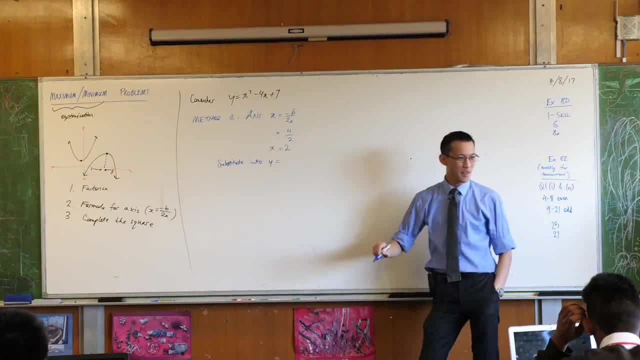 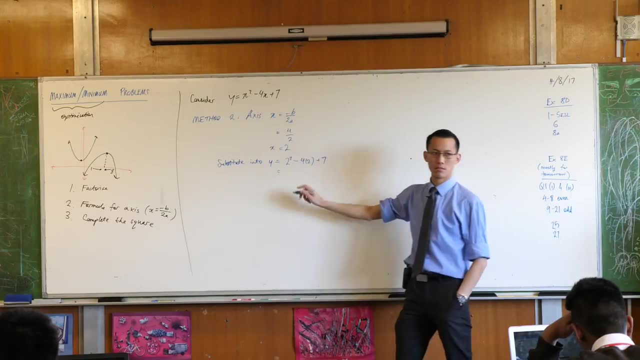 taking the hard way round for everything today. Substitute it into my top line: y equals two squared minus four. lots of two plus seven. Four minus eight plus seven, That's three. It's three right, Because this will become negative. four plus seven. 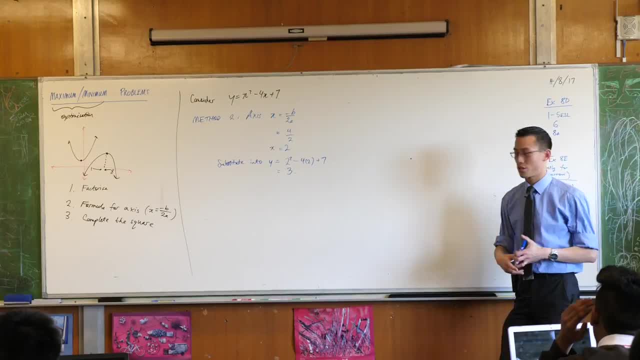 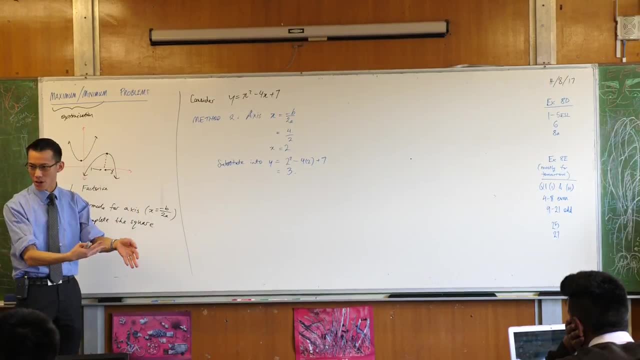 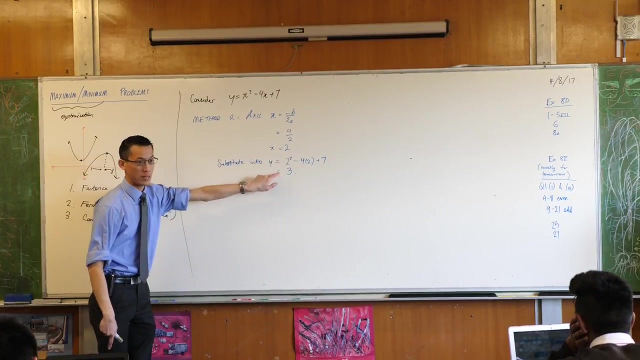 Ta-da, there you go. Okay. So in answer to the question, what is the minimum value? the minimum value is three, right? Where does the minimum value occur? It's when x equals two, So x equals two. that's not the minimum value. That's where you get the minimum value. 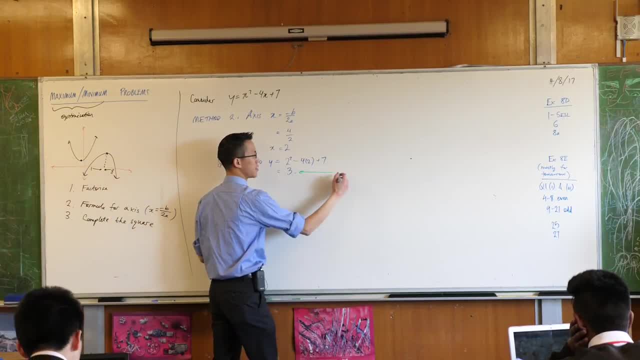 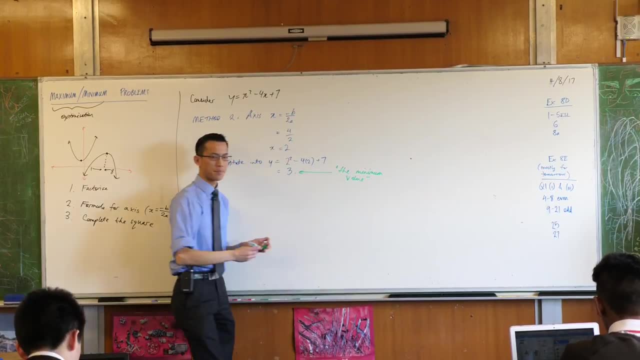 That's what this guy is, So maybe you want to label that This is the minimum value. Okay, So that was method two.